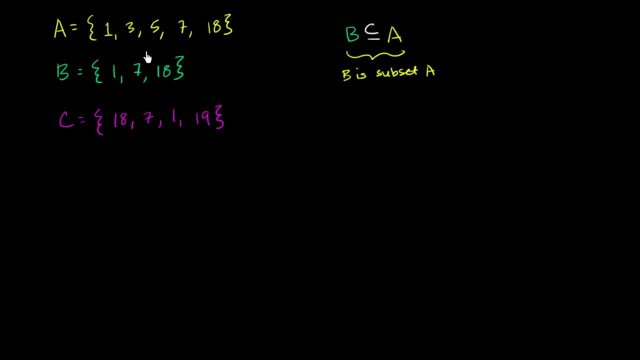 Because B is a subset of A, But it does not equal A, which means that there are things in A that are not in B. So we could even go further And we could say that B is a strict or, sometimes said, a proper subset of A, And the way you do that is you're. 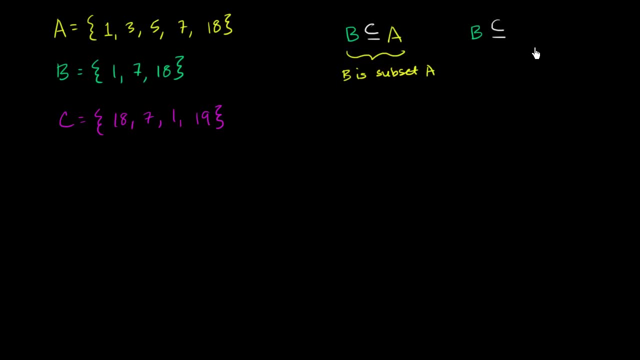 essentially you can almost imagine that this is kind of a less than or equal sign, And then you kind of cross out the equal part of the less than or equal sign. So this means a strict subset, which means everything that is in. B is a member of A. 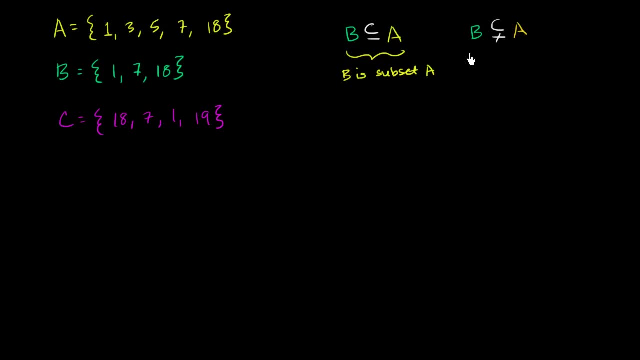 But everything that's in A is not a member of B. So let me write this: This is B. B is a strict or proper subset, So, for example, we can write that A is a subset of A. In fact, every set is a subset of itself. 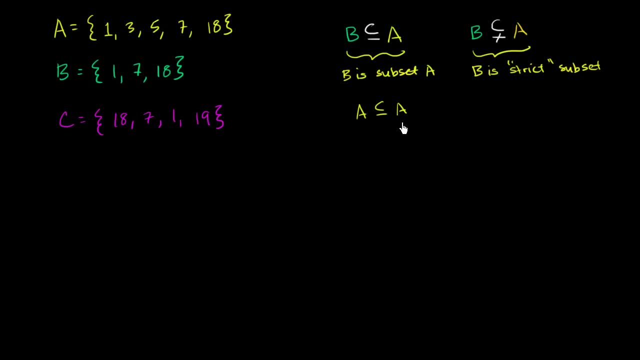 Because every one of its members is a member of A. We cannot write that A is a strict subset of A. This right over here, this right over here, is false. So let's give ourselves a little bit more practice. Can we write that B is a subset of C? 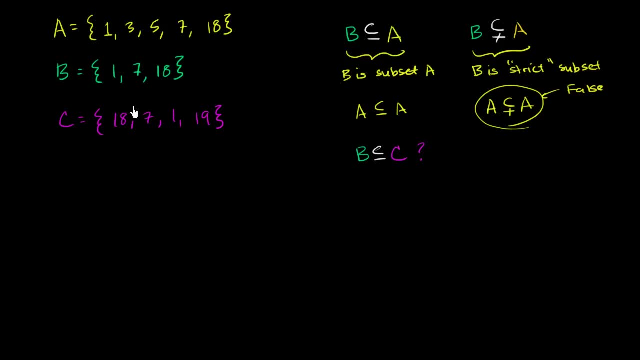 Well, let's see: C contains a 1. It contains a 7. It contains an 18. So every member of B is indeed a member of C. So this right over here is true. Now can we write that C is a subset. 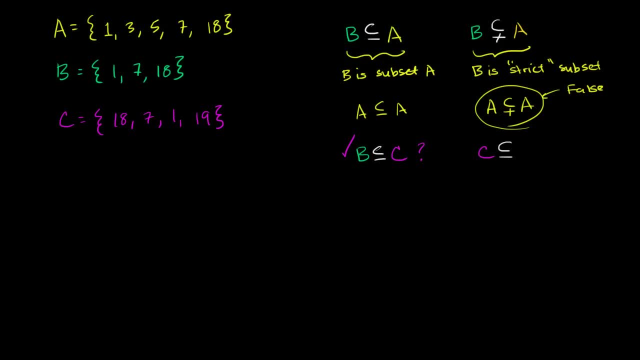 Is a subset of A. Can we write: C is a subset of A? Let's see, Every element of C needs to be an A, So A has an 18.. It has a 7.. It has a 1., But it does not have a 19.. 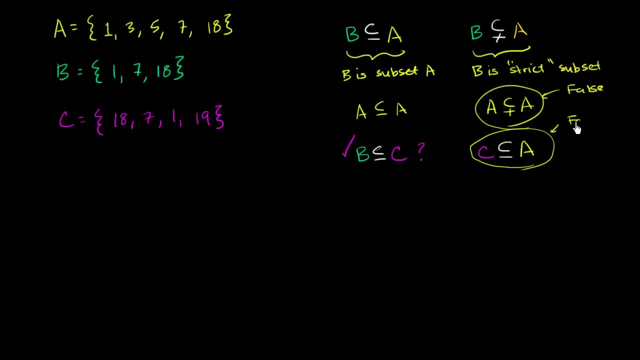 So once again, this right over here is false. Now we could have also added: we could write: B is a subset of C. Or we could even write that B is a strict subset of C- OK, Subset of C. Now we could also reverse the way we write this. 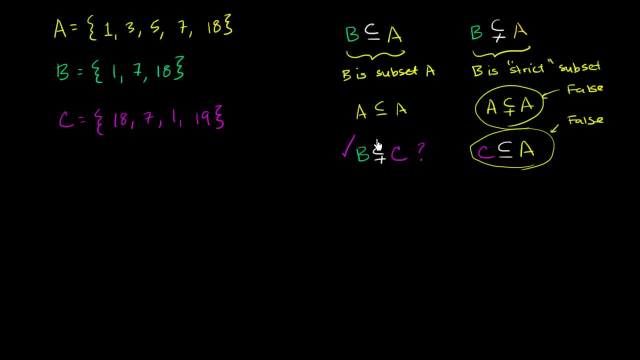 And then we're really just talking about supersets. So we could reverse this notation And we could say that A is a superset of B, And this is just another way of saying that B is a subset of A. But the way you could think about this,